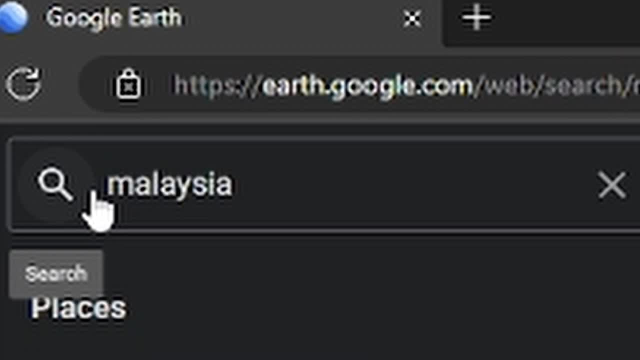 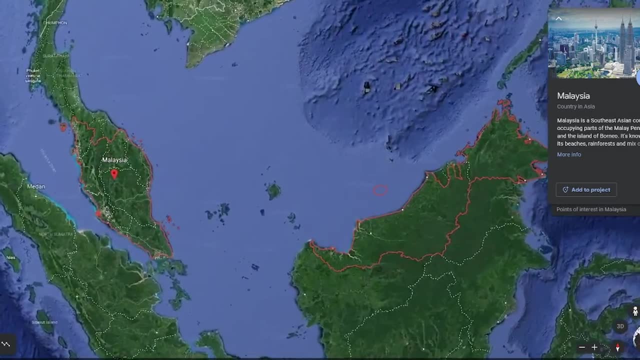 All right people, welcome to this channel where we discuss all things unfinished. See this, This tiny peninsular country. This is Malaysia. You might have heard of it, might not have heard of it, Doesn't matter, I'm gonna tell you anyway. So Malaysia is located in the Southeast Asia. 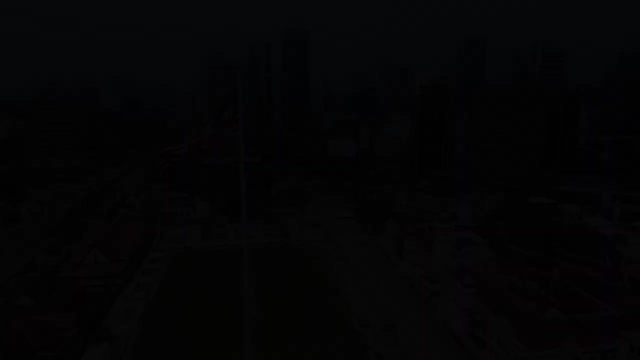 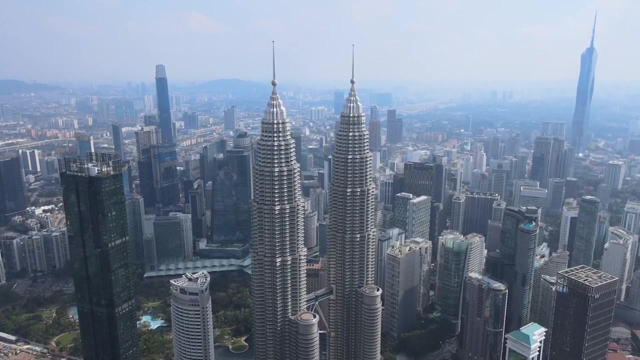 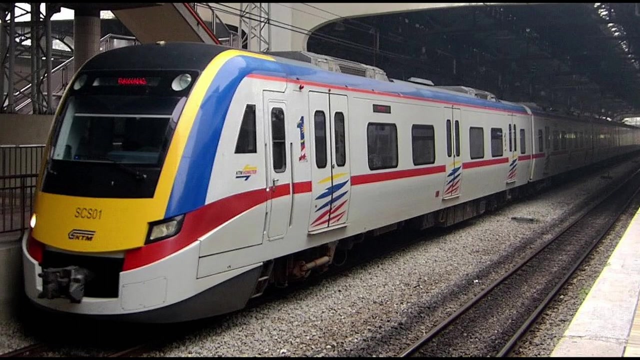 It has a population of about 32 million and more than 50% of its landmass is just forests. Its capital is Kuala Lumpur, and that's where we're going today, or more specifically, on its metro rail system. See, the metro rail system here came about in the early 90s when the economy was 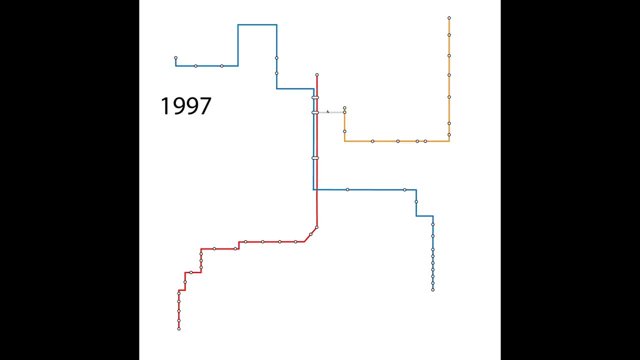 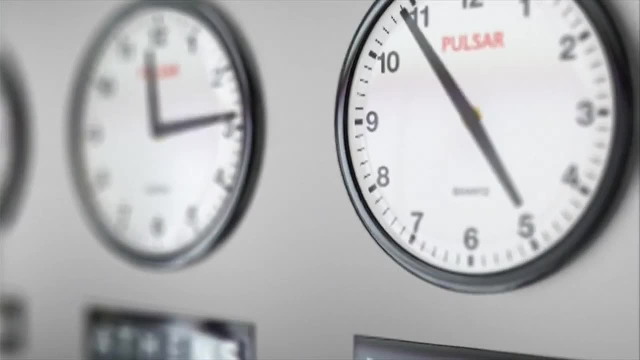 on a boom and traffic was starting to pile up. So the government planned a railway system throughout the city to carry people around and keep the roads clean of ****. So let's go back 27 years when it all started with the KPM. It's 1995 and traffic is bad. 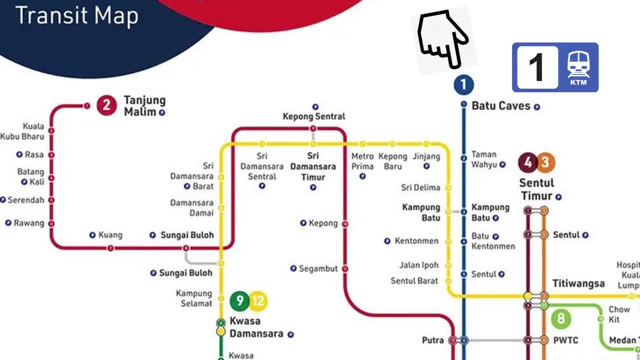 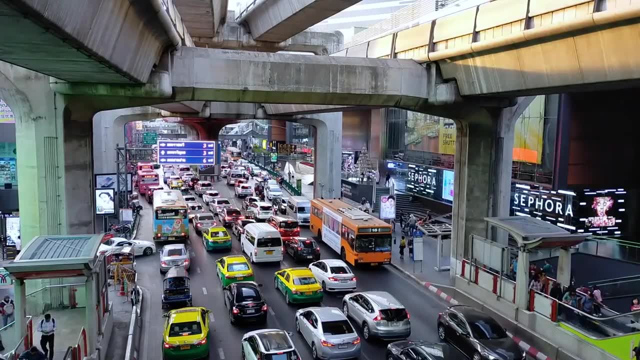 After the electrification of the Seremban line and the Port Klang line, the KTM commuter would begin its service carrying passengers from the suburbs to the city center, skipping the traffic altogether. KTM stands for Kerita Api, Tanah Melayu. The first service began with the Port. 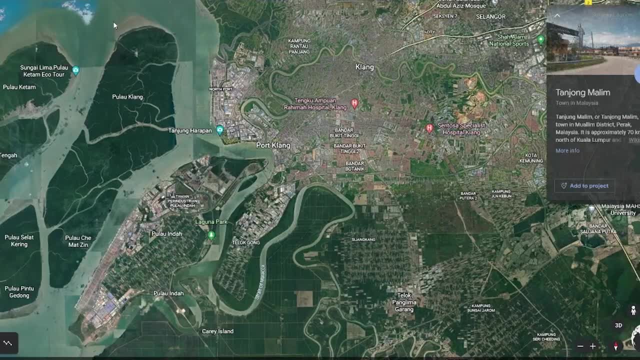 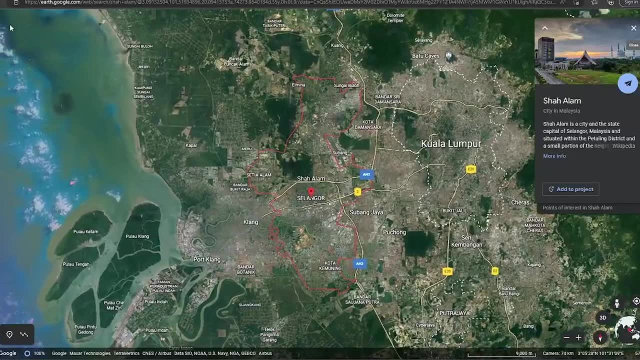 Klang line nearly 130 kilometers long, starting from Port Klang to Tanjung Malim. This line serves areas like Sungai Buloh, KL City Center, Petaling and Sha'alam. Majority of the areas this line serves are densely residential. 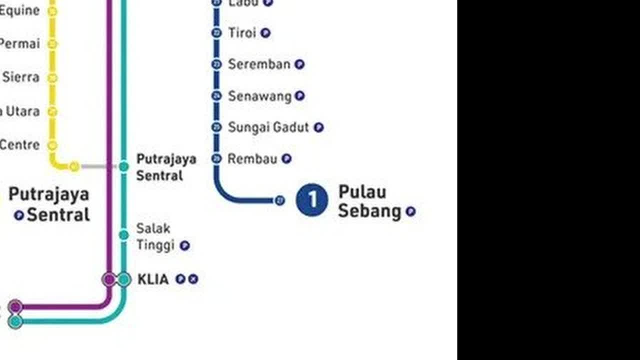 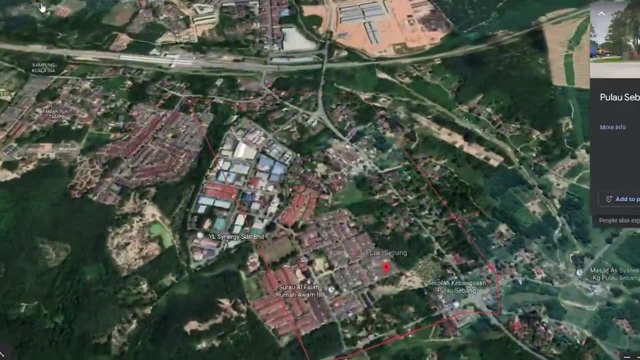 The second KTM line is a little longer, but not by much, but began as a spur line, 135 kilometers long, starting from Batu Cave to Pulau Sabang, And serves areas like Sentol, KL City Center and Kajang. 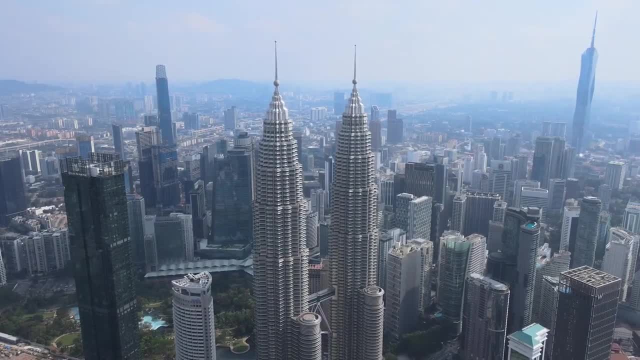 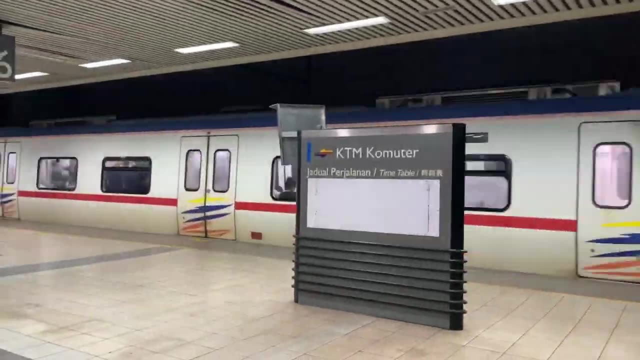 Again, majority are residential areas and city center. It also goes all the way to Seremban and Tampin, but those are in completely different states. Alright, onto the next one. Only 3 to 4 years later, the LRT would start its service Three lines. 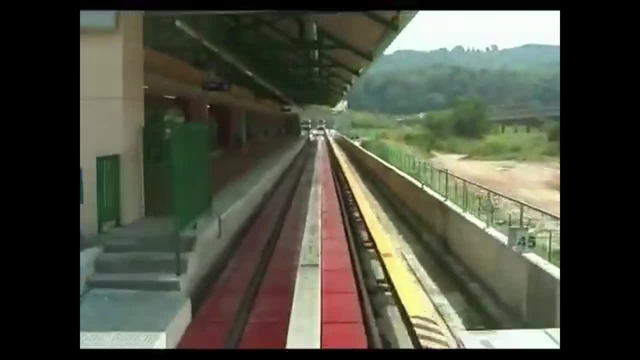 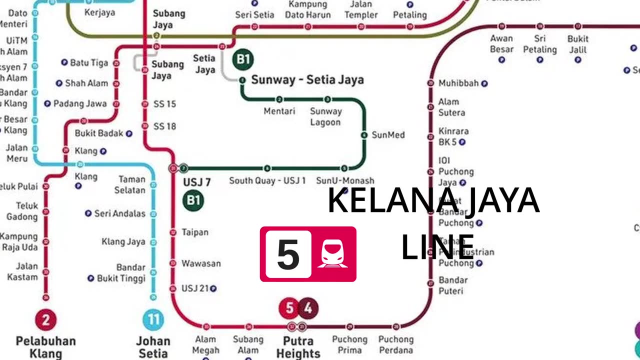 were constructed with the same purpose as the KTM Connect: the periphery to the heart, The Ampang line, the Seribu Taleng line and, a year after that, in 1999, the Klanajaya line, The first driverless. 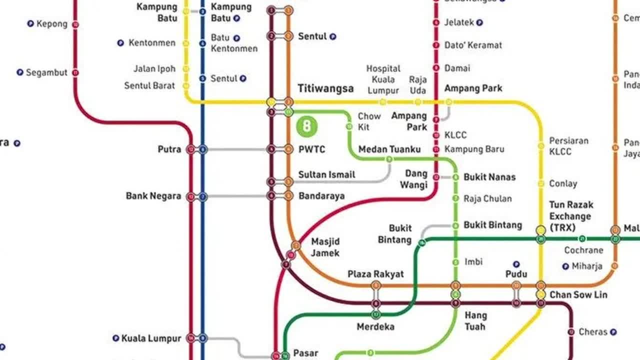 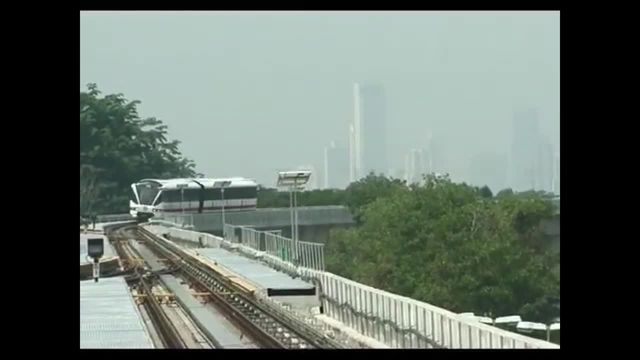 metro system in the country. The Ampang and Seribu Taleng lines were originally known as the Star LRT, First conceived as a transportation master plan concocted by the Malaysian government, But later, as companies like Prasarana and finally Rapid KL took over, the lines were renamed to Ampang and Seribu Taleng. 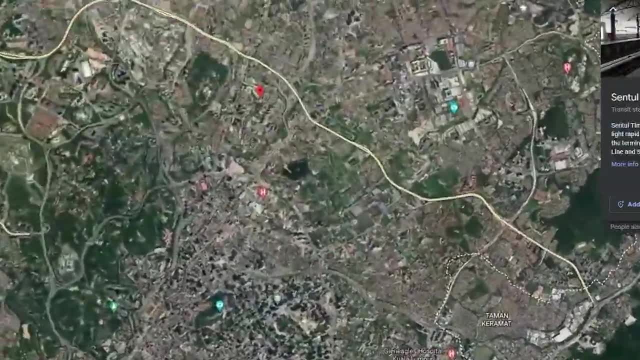 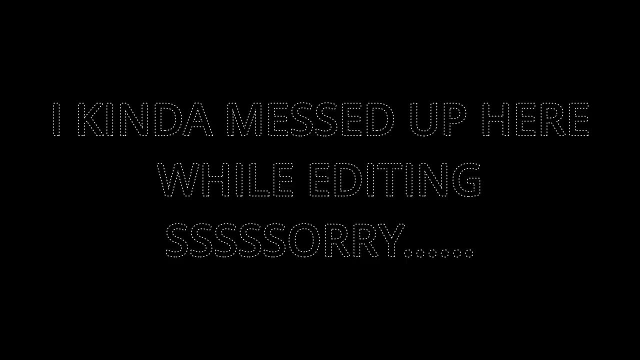 The Ampang line starts at Ampang and goes to Sentol Timur. This serves areas like Tiwangsa, Masjid Jamek and Plaza Rakyat, Basically very businessy areas. On the other hand, the Seribu Taleng line starts from Putra Heights and goes to Sentol Timur. 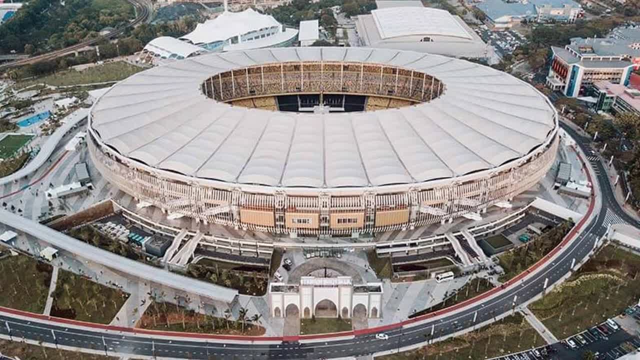 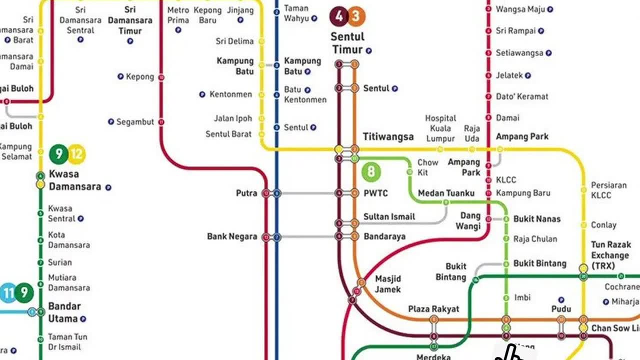 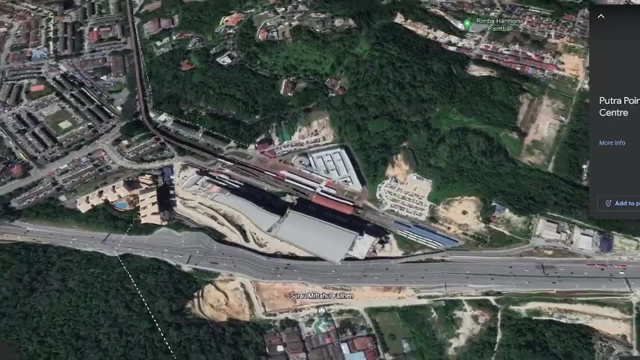 Serving areas like Bukit Jalil and Seribu Taleng. You might know Bukit Jalil as the biggest stadium here. Interestingly, both these lines share a common track between Chan Soh Lane Station And Sentol Timur station. Now the Klanajaya line goes between Gomba and Putra Heights, Where it connects to the Seribu Taleng line. 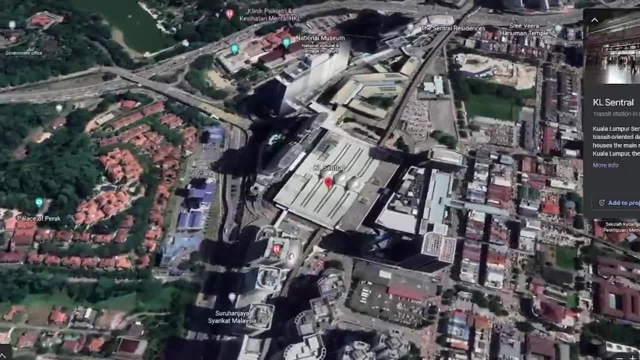 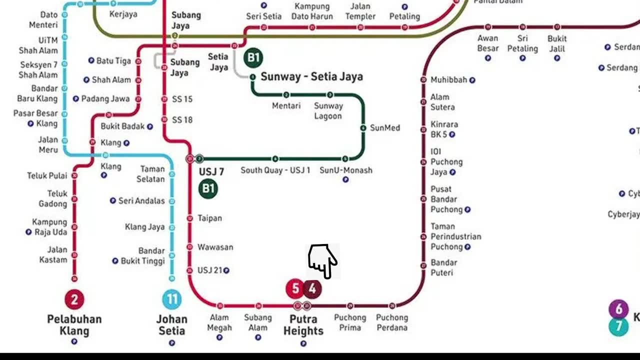 This line serves areas like KLCC, KL Central and University of Malaya. It goes through a lot of Kuala Lumpur's highest density areas. On the transit map, the Klanajaya line and the Seribu Taleng line might look like one continuous line. 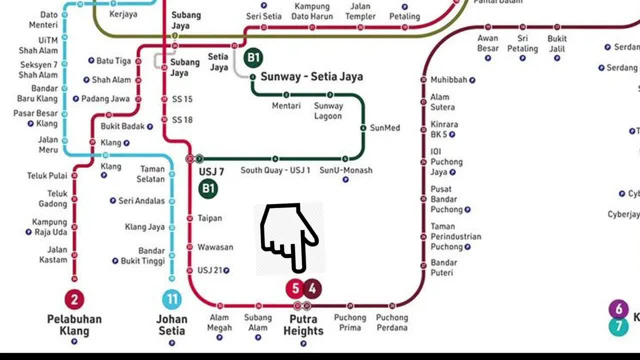 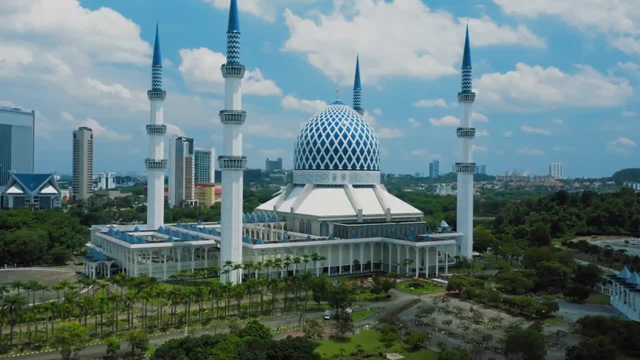 But in reality they're two separate lines and you will have to change trains once you get to Putra Heights station. There is another LRT line on the way And it's halfway through its construction construction: the Shah Alam line, which will serve from Bandar Utama to Johan Setia going. 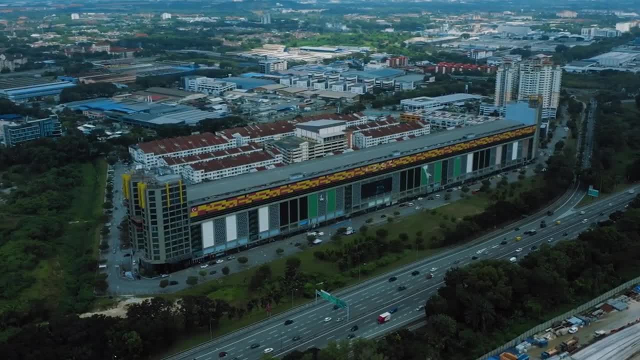 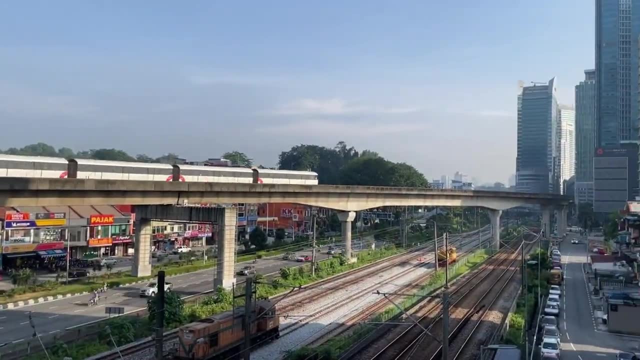 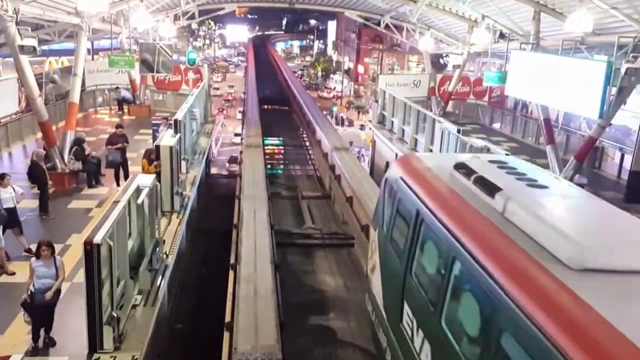 through areas like Glenmarie, Shah Alam Stadium and UITM University Right on to Kuala Lumpur's monorail. It basically serves as a people mover throughout the city center and the busiest commercial areas in the city, going from KL Central to Bukit Bintang. 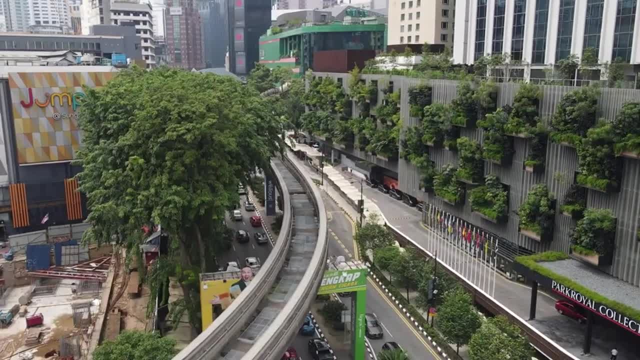 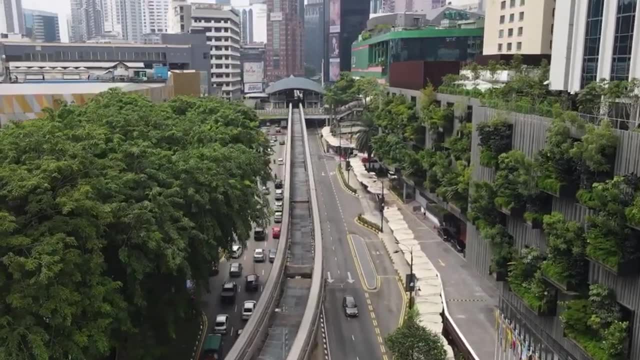 and terminating at Titiwangsa. The monorail scheme was announced by the Kuala Lumpur City Hall and, after a go-ahead from the Malaysian government, the construction began and in 2003,, it finally opened the single-tracked 8.6-kilometer-long loop through the heart. 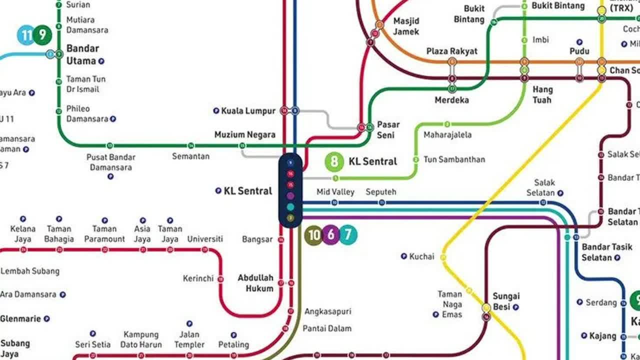 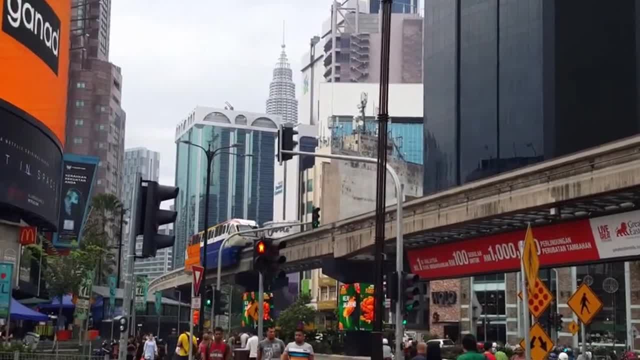 of the city. Initially, the plan was to have another branching line that would go towards Mid Valley and Abdullah Hukum, which would have integrated into the Port Klang KTM line, but was cancelled due to the 1997 Asian financial crisis. There is, however, a new line in the 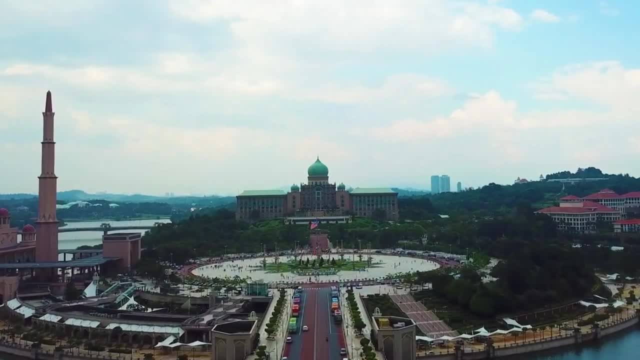 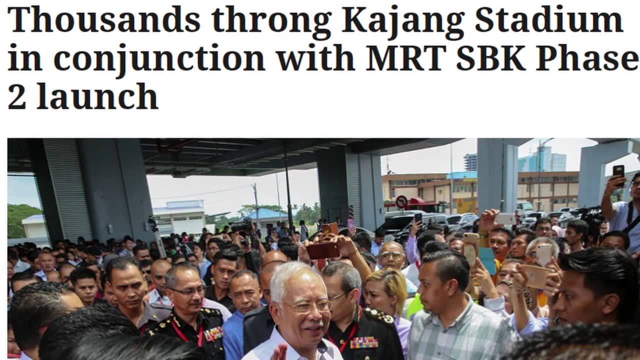 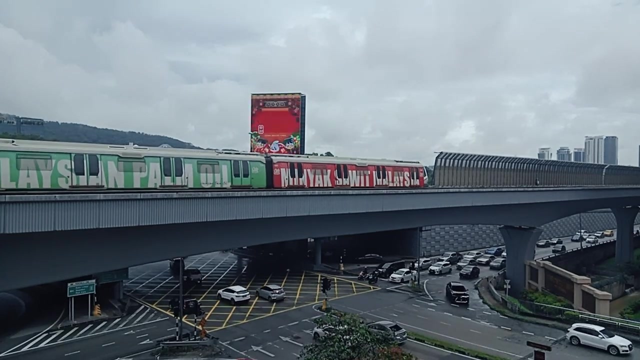 plans for Putrajaya, although it's tough to say when it will be finished, considering that the construction has been stalled since 2004.. In 2016,, the Malaysian government launched a whole new system of trains, the MRT lines, or the Mass Rapid Transit line. The first of them started full service on the 17th of 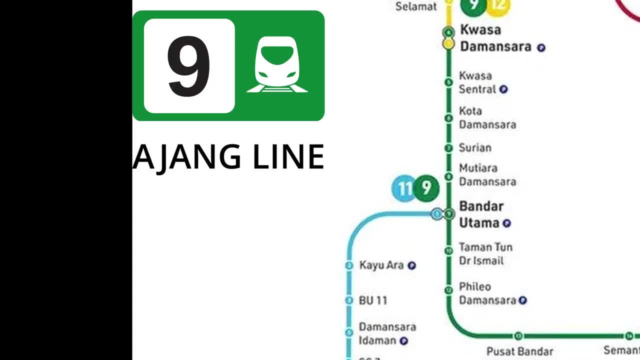 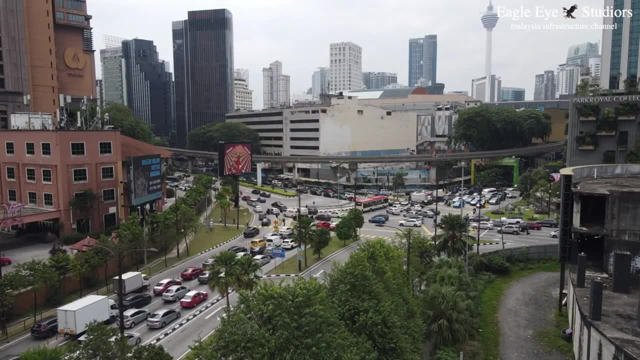 July 2017.. The Kajang line serves from Kwasa, Damansara to Kajang, going through areas like Banda Utama Museum, Nigara and Bukit Bintang. The second line, the Putrajaya line, was launched in its first phase last year, but has yet 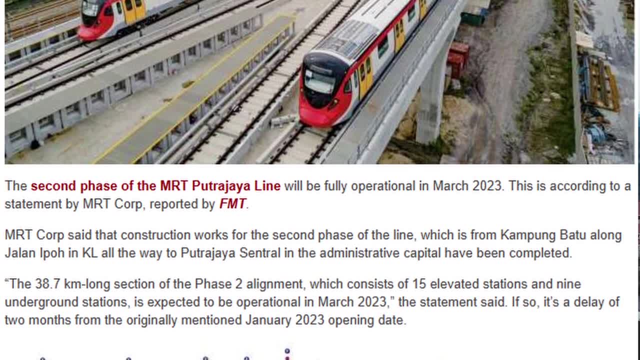 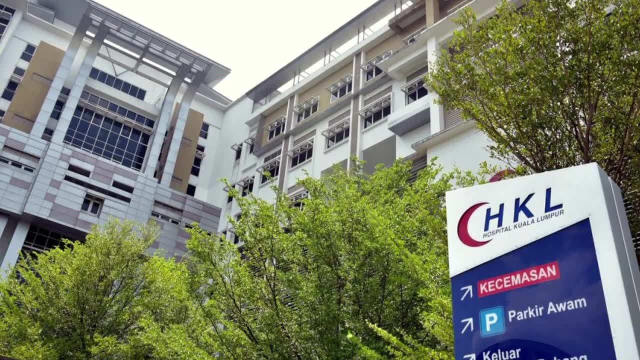 to be fully operational, which is set to be this year. Once it is fully operational, the service will span from Kwasa, Damansara to Putrajaya Central, serving areas like Kuala Lumpur Hospital, KLCC, UPM University and Cyberjaya. There is a third upcoming MRT line. 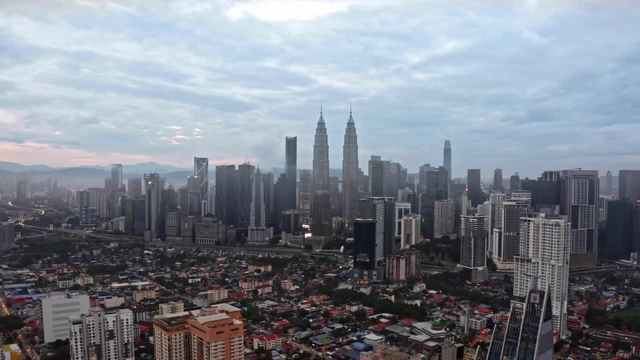 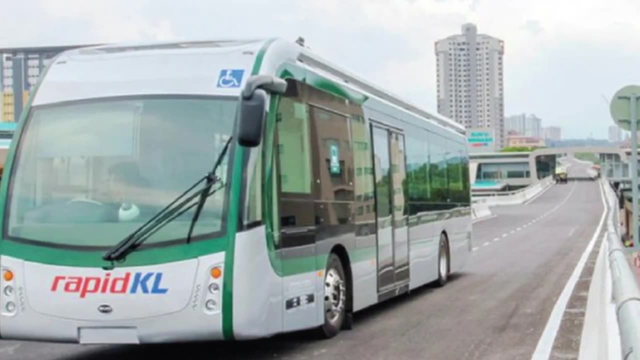 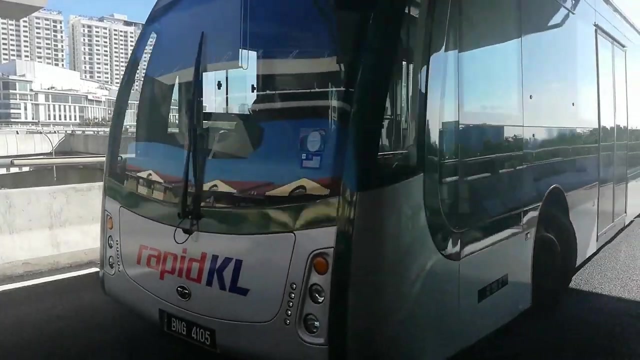 which has been approved. The Circle line will serve in a loop around the city without entering the business district. The Sunway BRT line serves only in the Sunway area, from Sunway Sityajaya to USJ7.. And a little bit of trivia: this line happens to be the world's first all-electric BRT line. 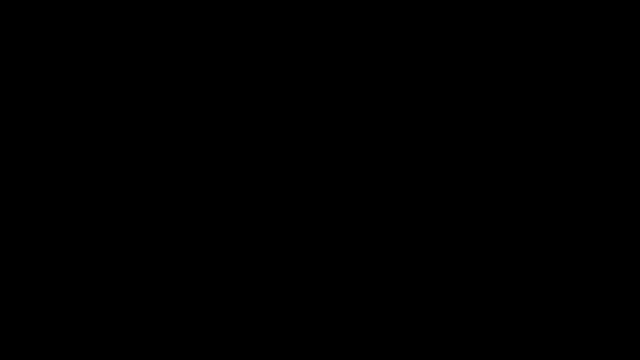 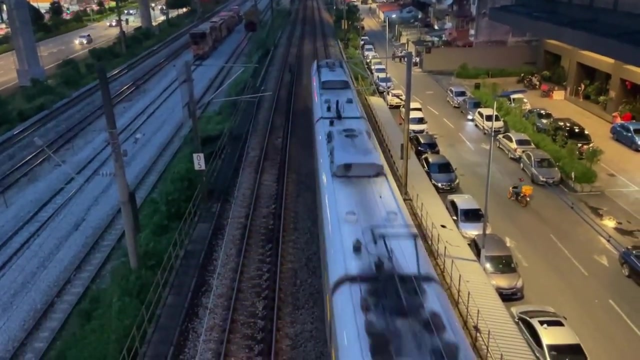 serving only about 7 stations. So now, after all of those, there are still three airport rail links left to talk about, one of which serves more like a transit train. The KLIA Express, or the Kuala Lumpur International Airport Express, is the first of its kind. The KLIA Express, or the KLIA Express, is the 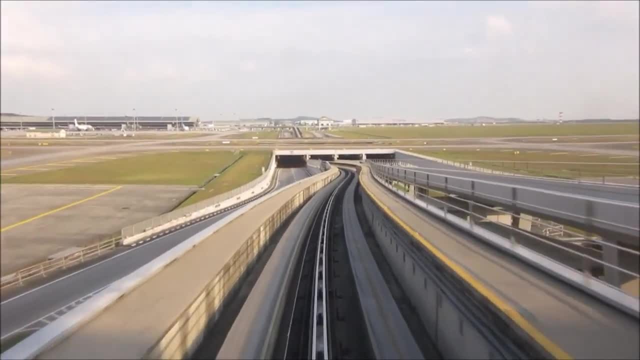 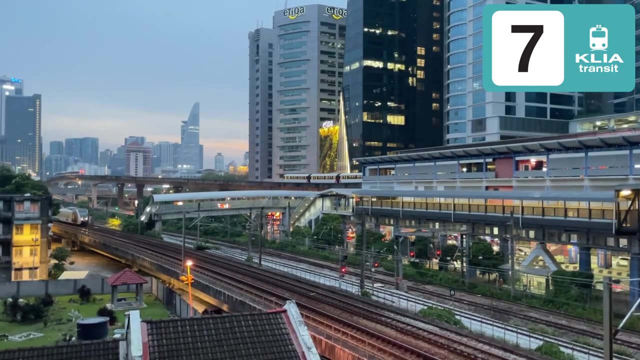 first of its kind. The KLIA Express goes directly from KL Central to Kuala Lumpur International Airport, And the Skypark rail link goes directly from KL Central to Subang Airport. The KLIA Transit, however, goes from KL Central to KLIA, but stops at stations like Putrajaya. 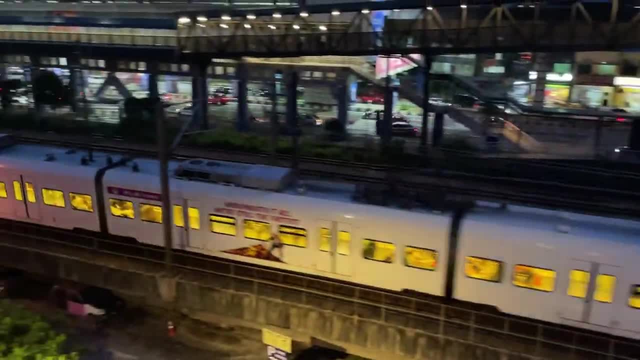 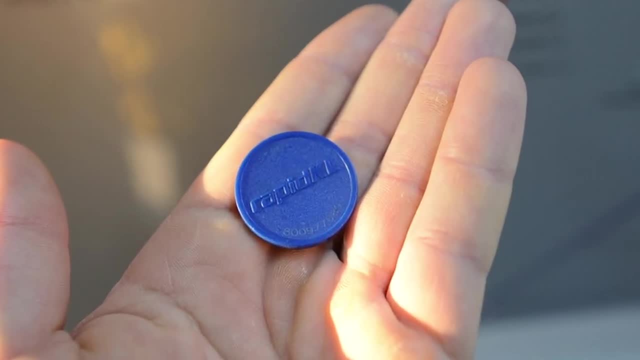 Central and Banda dasislatan. All of this combined forms the Klang Valley Integrated Transit System. So how do you access it? Well, you can either buy tokens, which are available at ticketing machines at every station, Or you can also get your money from a local token, or you